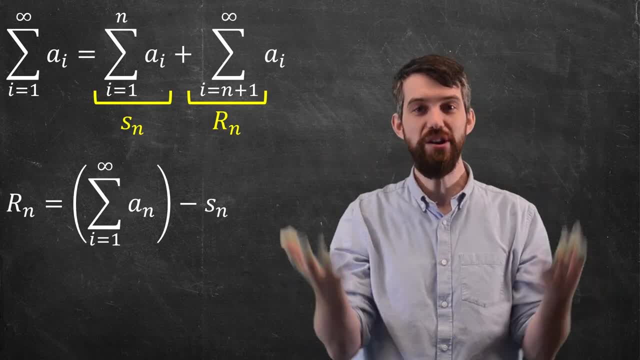 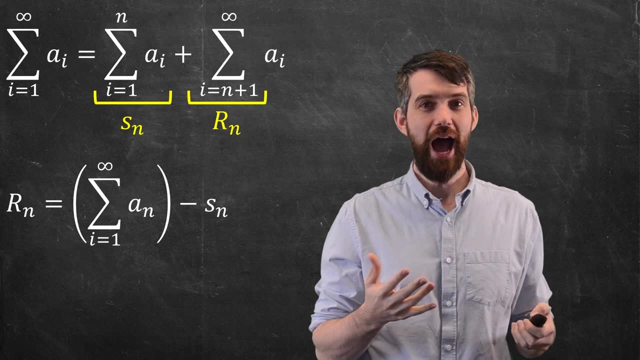 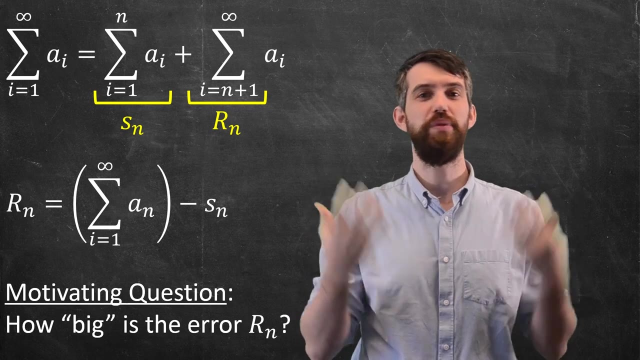 one more time. Let's say we wish and we can say that the remainder term is the entire series subtracted off the partial sum. So the question that's really going to motivate us is how so-called big is this error term, this remainder term Indeed? imagine you go and you compute out S10. 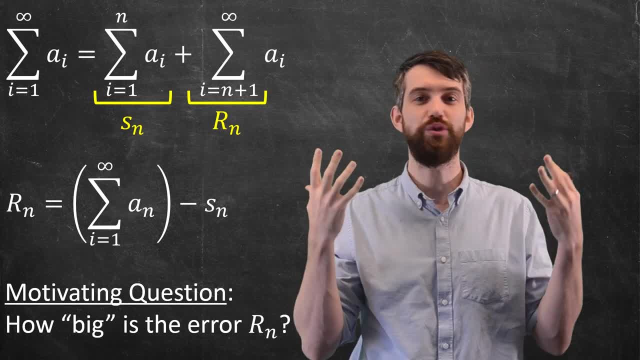 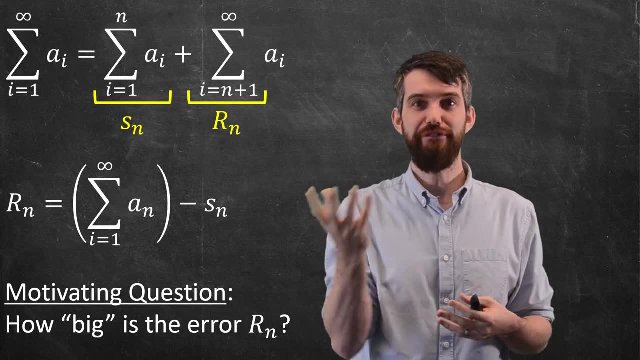 or S100, or you have a fast computer and you compute out S1 million. You add up the first million terms. A computer can do that. So then the question is: you've got some value, and is that value really close to S1 million? Is that value really close to S1 million? Is that value really? 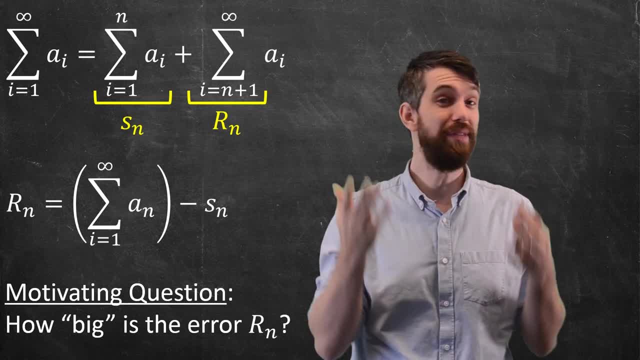 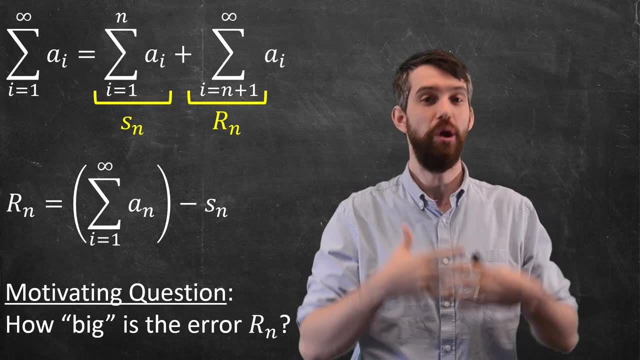 close to the thing it converges to or is it really far away? And indeed the answer to that question might depend on your specific discipline and what the standards and uncertainty that you're allowed to have in your specific discipline. But we're going to try to come up with some formula. 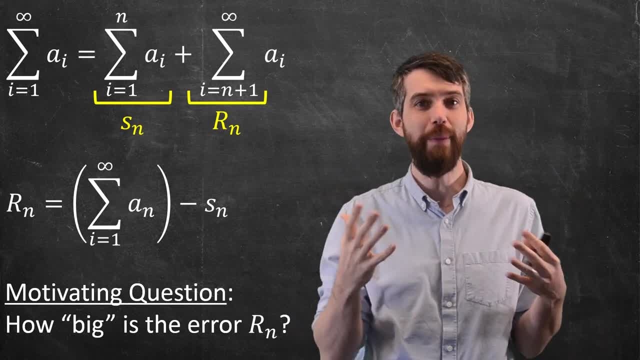 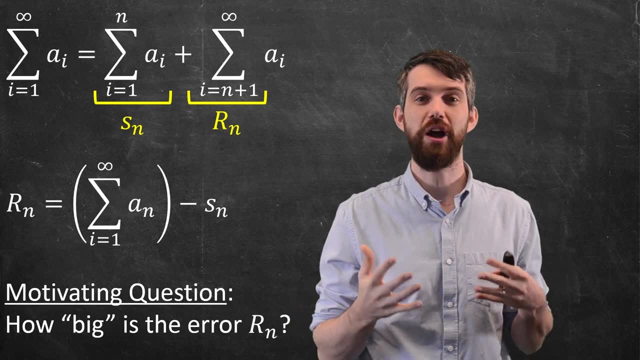 that tells us how bad is this remainder term, How bad is our estimate going to be if we approximate by just taking, say, the 10th partial sum? Now, the way we're going to talk about this is quite related to the integral test. Indeed, I want you to consider some function that I have here in f of x. 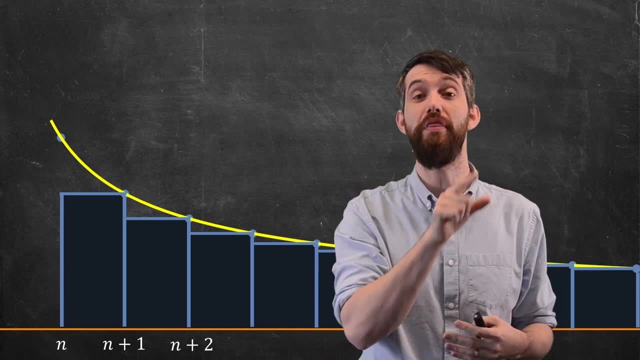 I'll have a course. I'm going to have a course on the corresponding sequence, which gives me points on that curve. Notice, by the way, that I haven't put the y-axis on the graph. I'm starting some ways out. I'm. 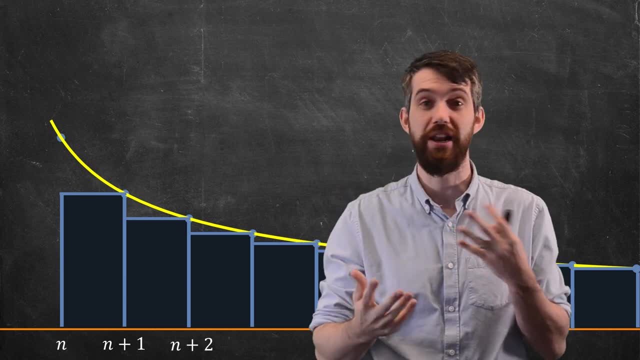 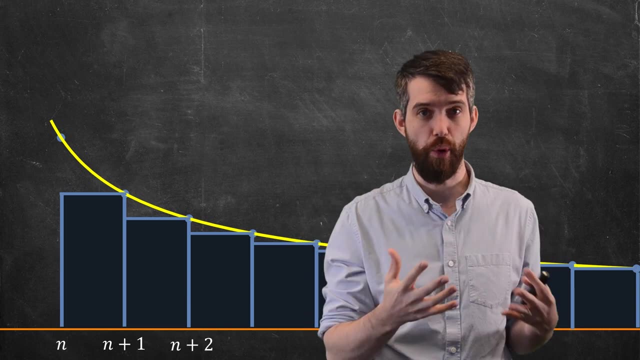 starting at n, and then I'm going n- n plus 1,, n plus 2, and so on. I haven't shown you anything between 1 and n. I'm only showing you n and so on. Now for these rectangles, I'm going to use a. 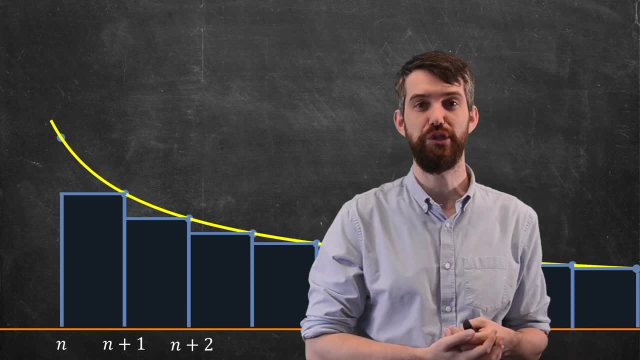 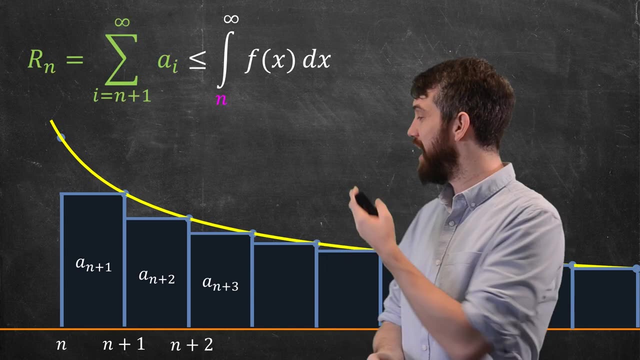 right endpoint to define the height of them. So, on the interval from n to n plus 1,, the height of this is going to be a n plus 1.. The width is 1.. is that the area of the first rectangle is a n plus 1,? 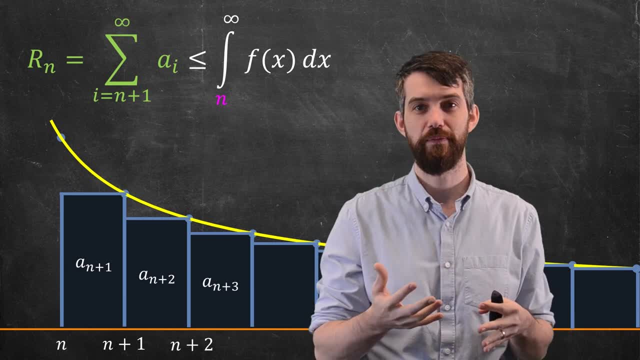 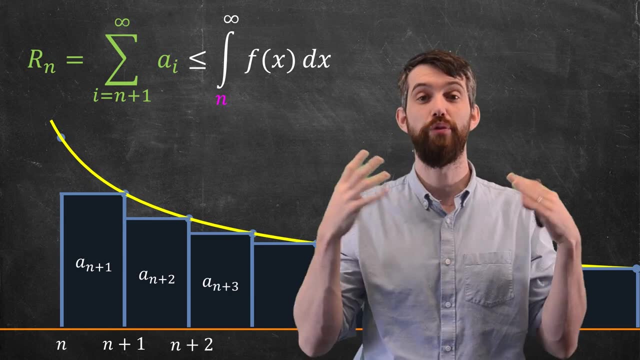 and the second one is a n plus 2, a n plus 3, and so on. So now what I have is this relationship between this geometric concept and my series. I can talk about the remainder, which was the series, but from n plus 1 up to infinity, that's the area of the rectangles. 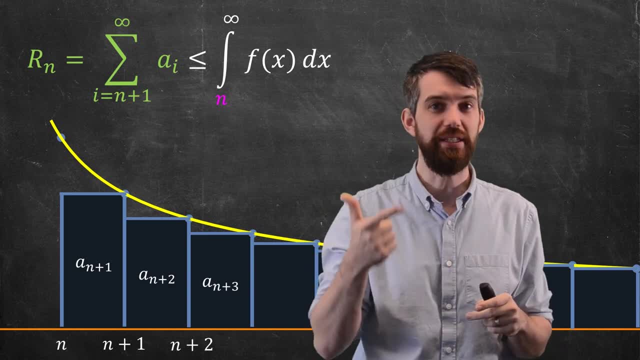 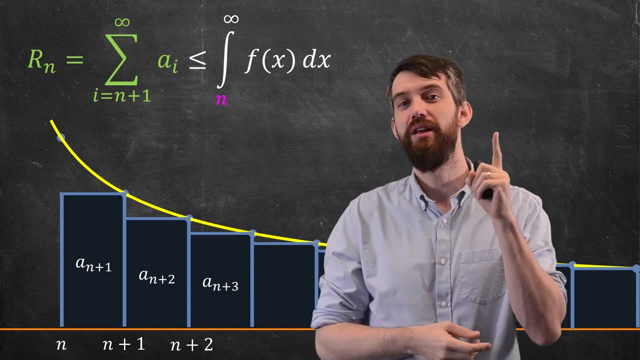 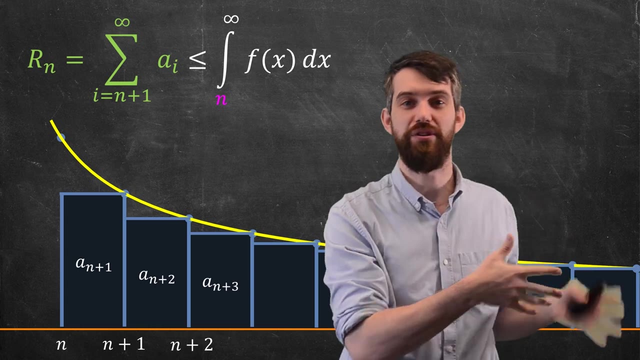 And the way I have drawn it with this positive, decreasing and continuous function, is that the area of these rectangles of the remainder is less than the improper integral from n up to infinity. So I have an equality here. Okay, I want to do the same trick, but on the other side. 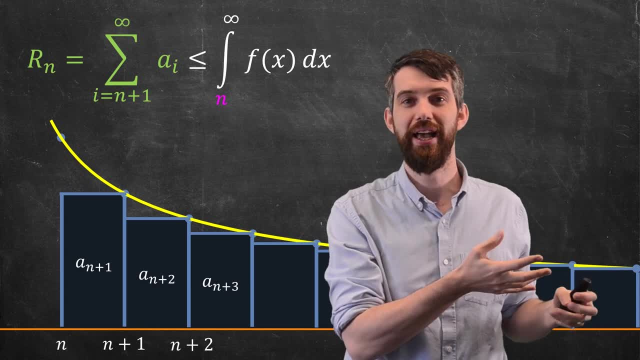 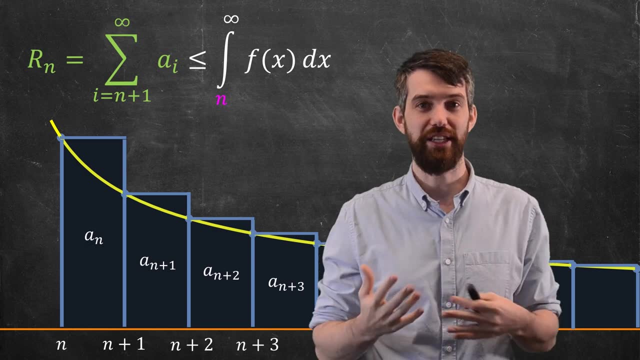 to get a different inequality to bound the remainder in the other way. So now, what I'm going to do is not this, but I'm going to do left endpoints instead. And what this does, if I do left endpoints, it makes all of my rectangles bigger. 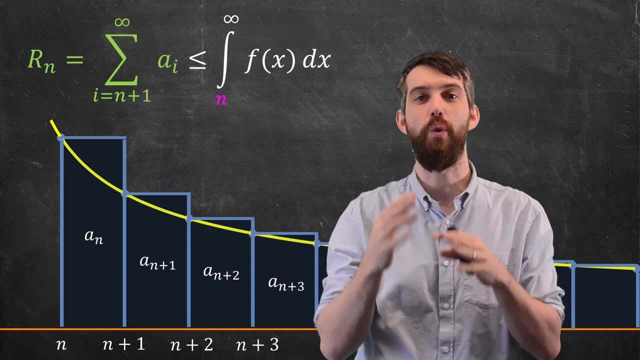 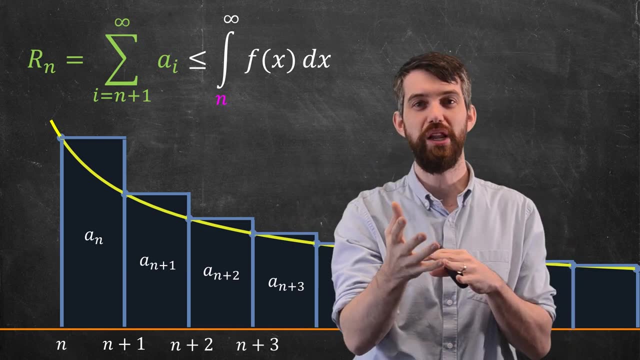 The first one has an area a n, the second one a n plus 1, its third a n plus 2, and so on. But if I look at my remainder formula, my remainder formula only starts at a n plus 1.. 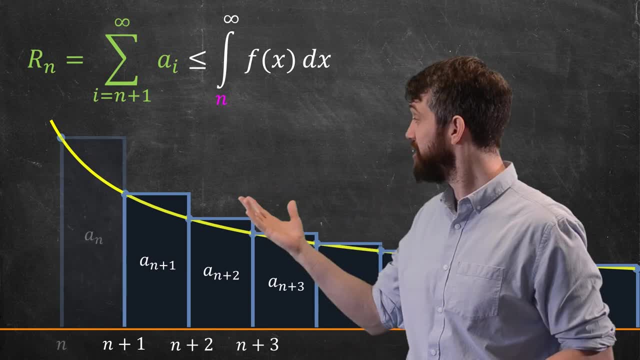 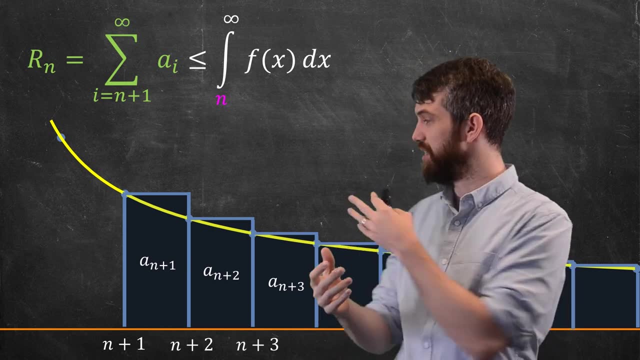 So this first rectangle that I've drawn, the one with area a, n, let's just get rid of that entirely, because I just don't care about that. I care about starting at a, n plus 1.. But now, if I look at this series, 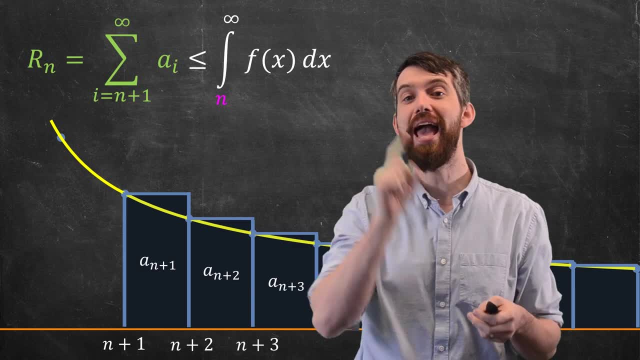 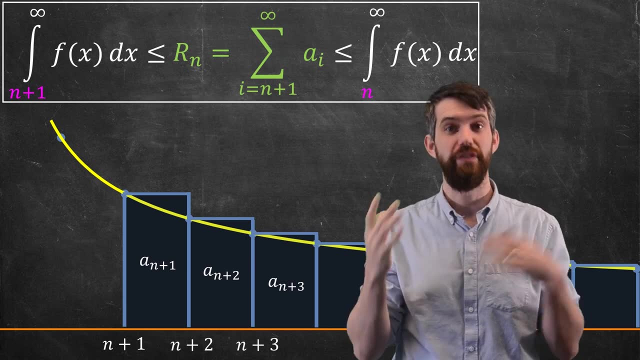 this series is all bigger than the integral, starting at n plus 1 up to infinity. So I have an inequality on the other side, namely that this remainder, your term, is bigger than the integral, from n plus 1 up to infinity. So it's, in a sense, squashed. 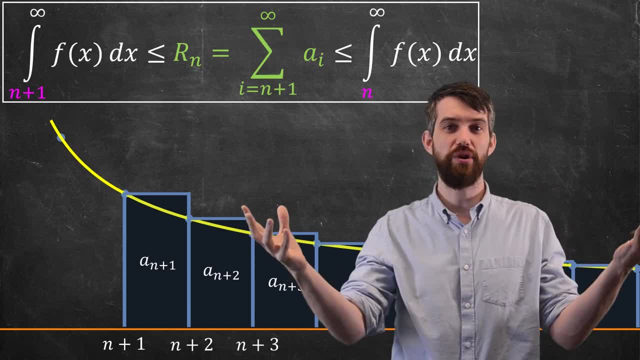 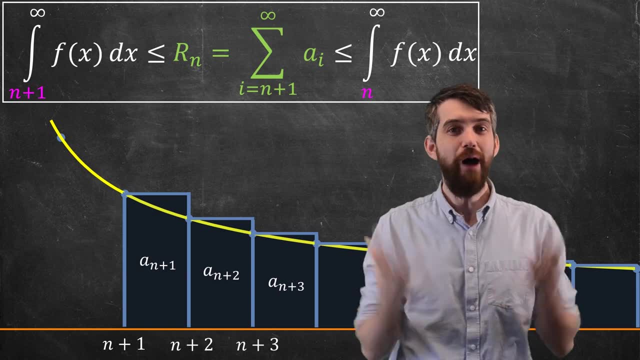 It's got the integral from n plus 1 up to infinity on one side, the integral of n up to infinity on the other, and the remainder sits there in the middle of it. So this is a bound. It tells me how bad could my remainder be? 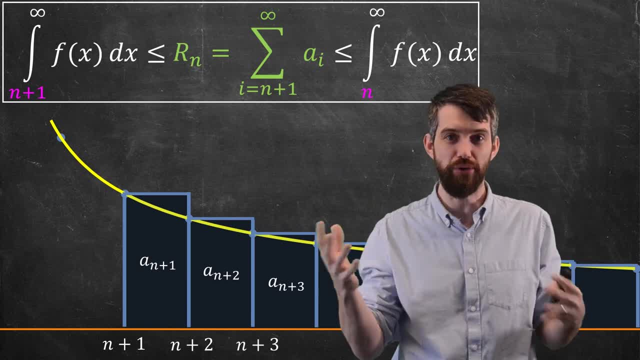 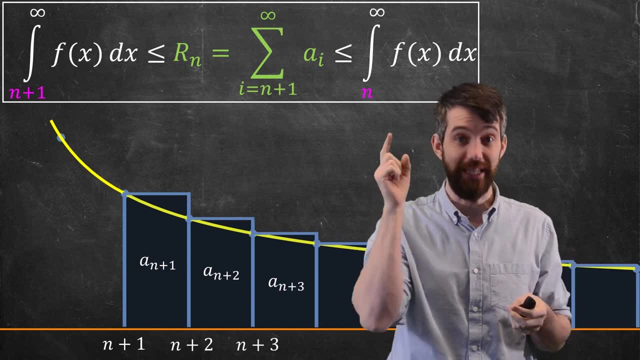 Well, it has to be bigger than and less than these two different intervals. So if I want to estimate on my remainder how bad it might be, I can compute these intervals, and that doesn't tell me what my remainder is exactly, But it gives me a reasonable bound that I can use. 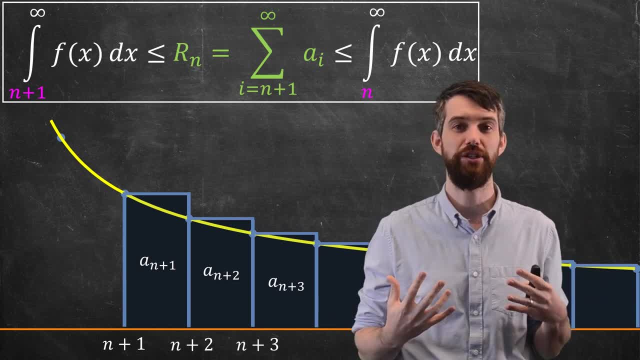 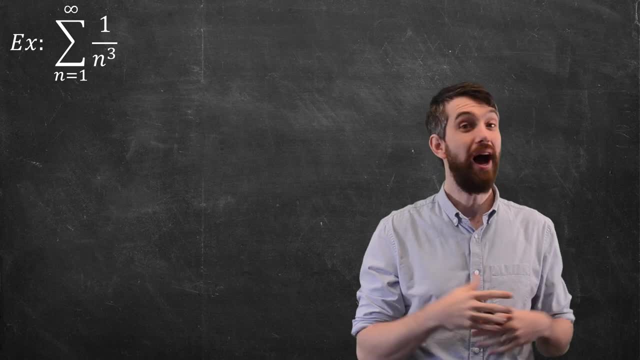 to see whether my estimation is good enough for my particular application. So, as an example, let's consider this series: the sum from 1 up to infinity of 1 over n cubed. Now I know the series converges. Indeed, if we go back to the first video on the integral test. 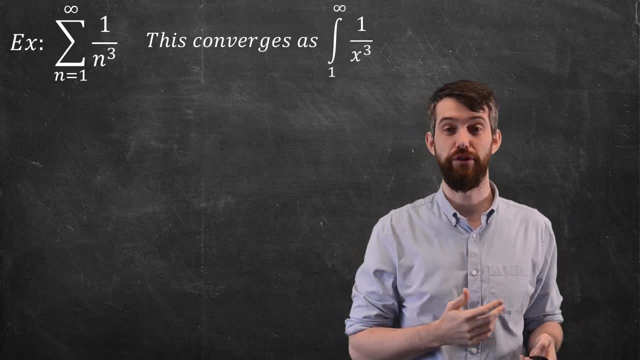 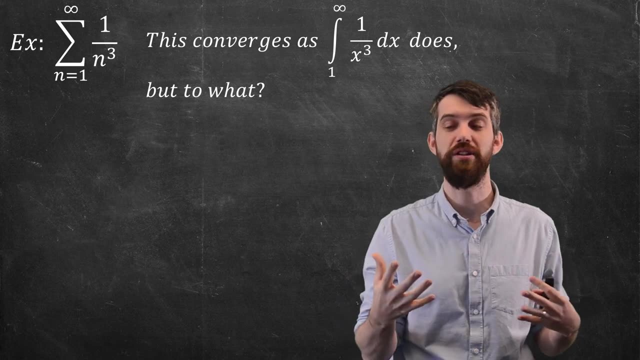 this is just a p-series, and the p-series converges here because I relate it to the p-integral 1 over x cubed, where p- the 3 here- is greater than 1.. And so that we know, this improper interval converges and so too does the series. 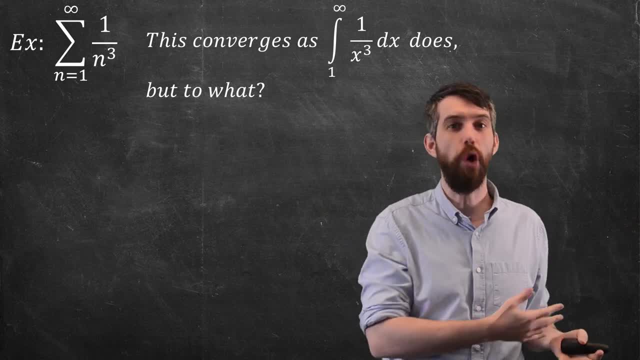 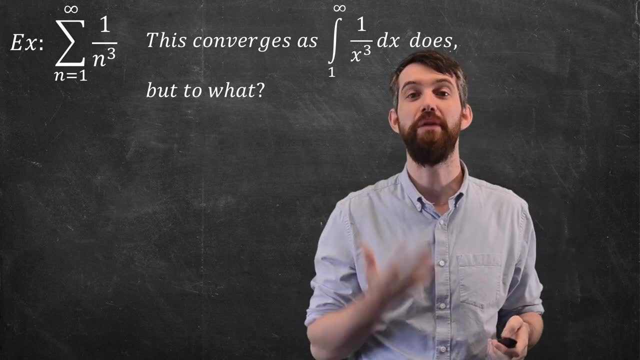 But what does it converge to? We don't know. The integral test only tells us does it converge or does it diverge. It doesn't tell us what it converges to. So let's suppose we go away and we compute the value of s10. 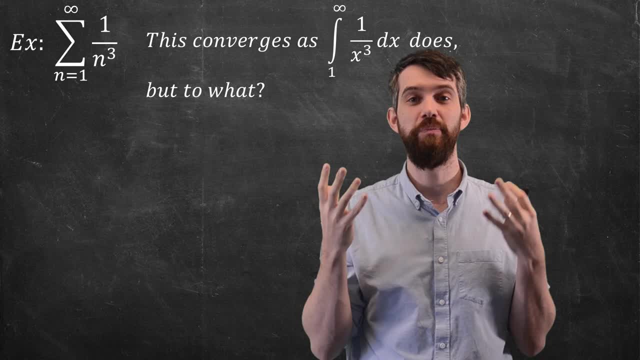 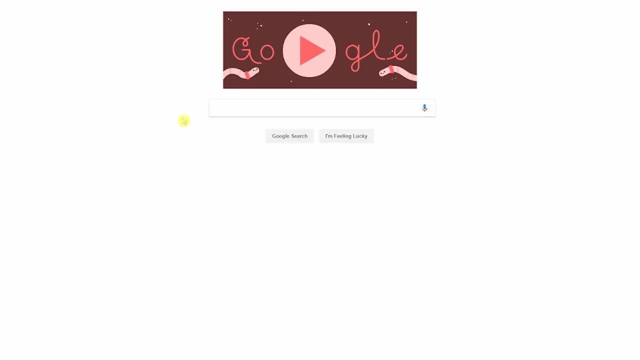 Okay, so let me say that we go away and we're going to compute manually, via a calculator, via a computer, the answer to s10, the 10th partial sum To compute this value of s10,. I'm going to go to a very useful website, which is WolframAlpha. 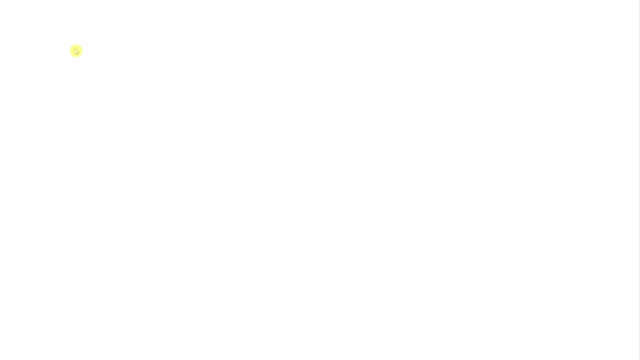 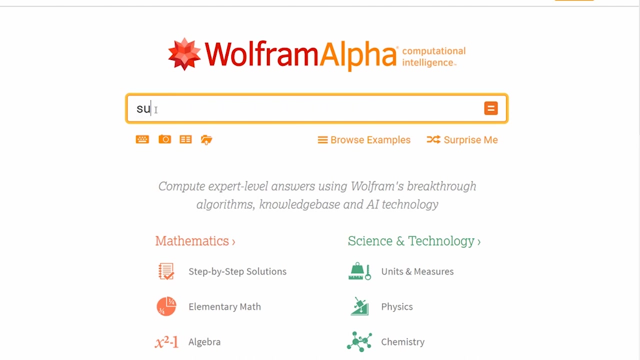 And WolframAlpha is that calculator on steroids that allows you to compute an enormous number of things And it interprets what you say in a relatively clever way. So, for example, we want to do the sum, And we're doing this from the value of 1 up to 10,. 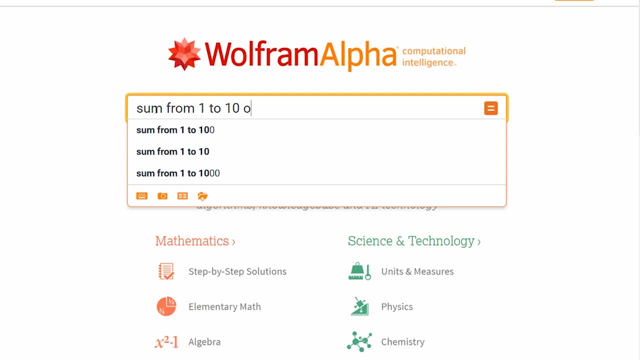 if I want to figure out the s10, the 10th partial sum, And then of what function am I doing? 1 over n cubed? I hit enter and it's going to go away. It's going to think about it for a moment. 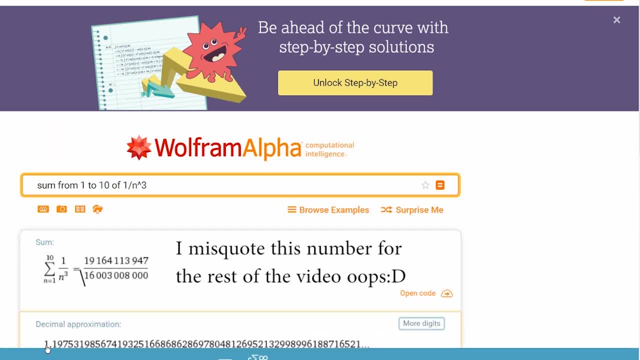 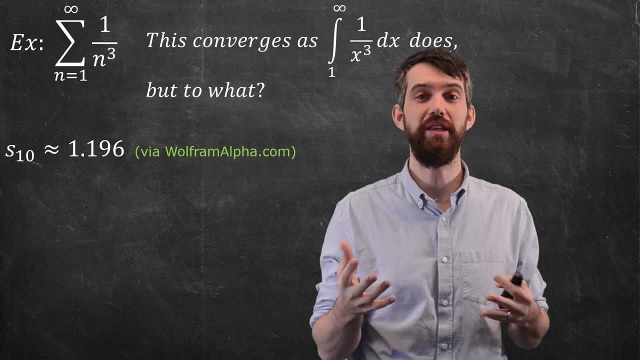 And it spits out that the value approximately is 1.198.. And so that is the value that I'm going to use for my s10.. So we've gotten this approximation: s10 is approximately 1.196.. Now what about the remainder? 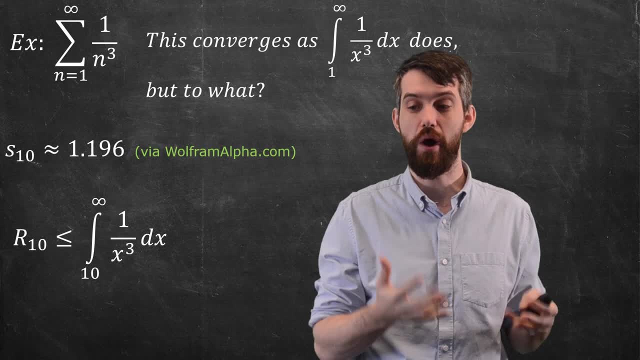 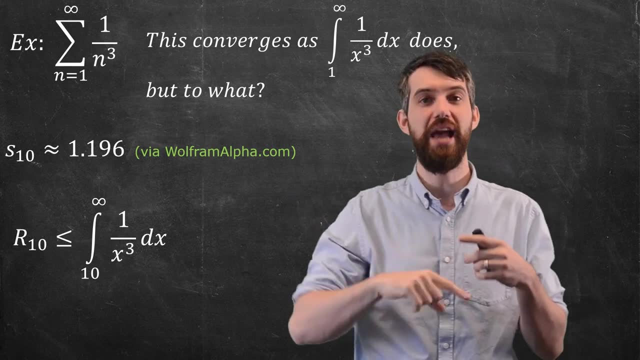 So, by this business of comparing it to an integral, the formula we've gotten is that r10, the remainder, when you take 10 terms, is something smaller than the integral from 10 up to infinity of 1 over x cubed dx. 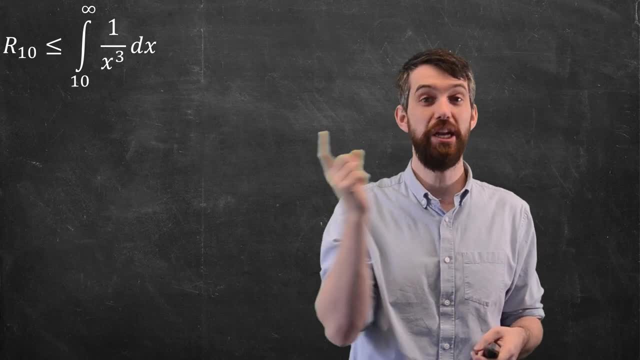 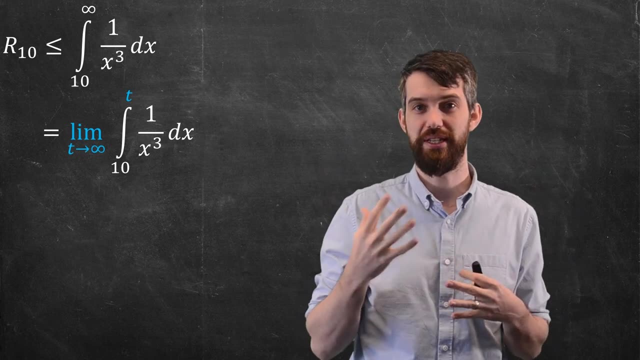 So we can do that integral. So let's just go and consider just that integral First. it's an improper integral. So instead of the infinity, I have to pull it out and talk about a limit, as t goes to infinity, where I've got this integral from 10 up to t. 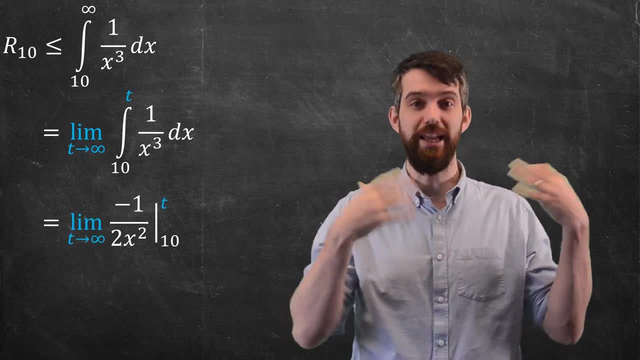 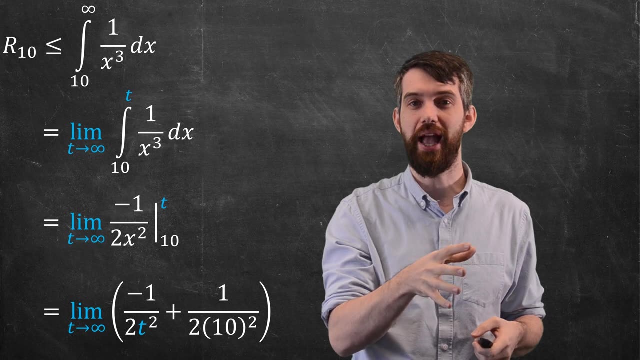 I can do this particular integral. it's just a power rule. So I keep the limit out the front and I integrate it. I get minus 1 over 2x squared. I'm going to plug in the t. I'm going to plug in the 10.. 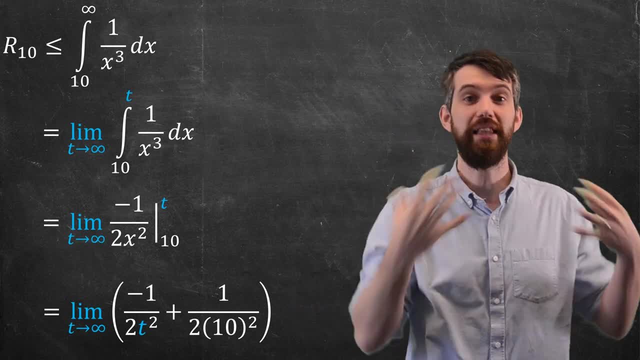 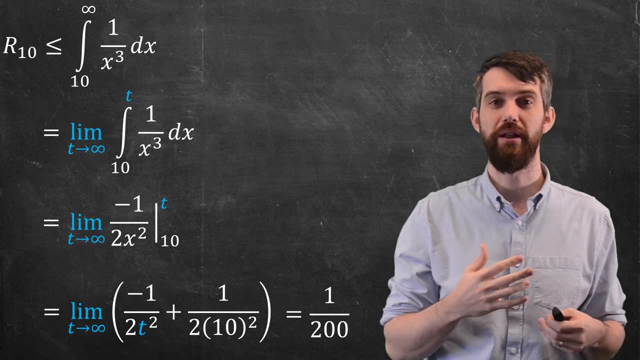 And then because the t is in the denominator, if I take the limit as t goes to infinity, the first term goes away. I'm just up to the second, That is, I just have 1 over 200.. So that tells me a bound on my error. 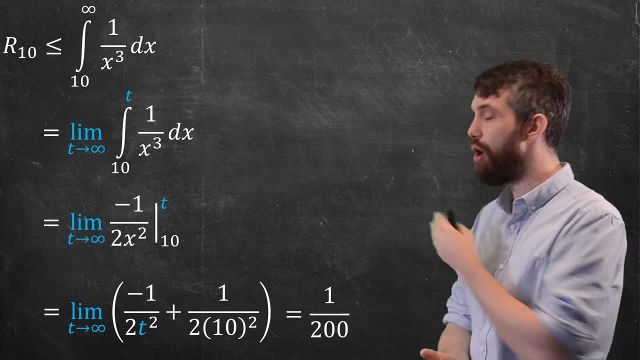 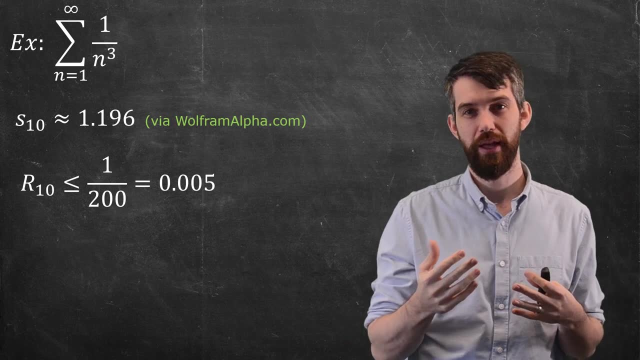 The remainder is something smaller than 1 over 200.. So what do I know? I'm beginning here with this example: the series that is adding up 1 over n cubed. I have done the s10, so my approximation by adding 10 terms. 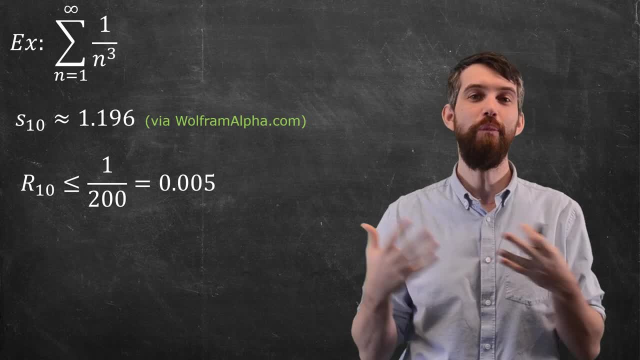 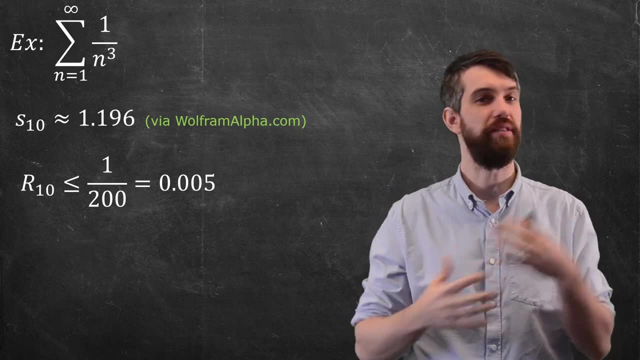 I've gotten the value of 1.196.. And then I asked how bad is my remainder? and my remainder is less than 0.001.. Now, my series is one of these positive decreasing ones, the requirement that makes all of this stuff work.